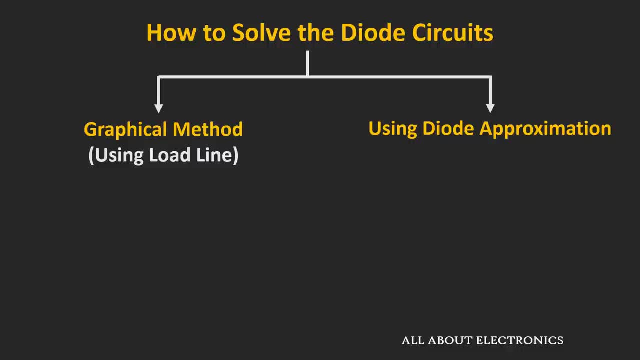 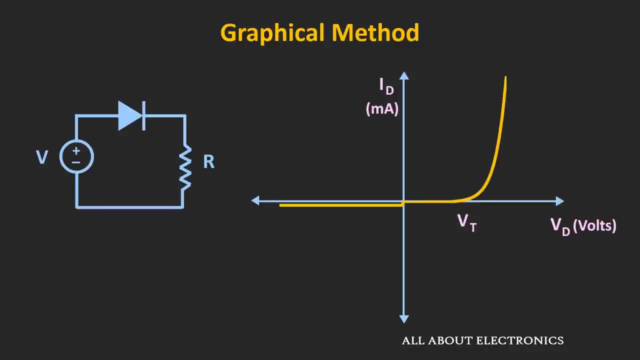 And the second method is the diode approximation. So first let's see how we can solve the circuit using the graphical method. Now, like I said, in this graphical method, using the load line, we can find the voltage and current across the diode. 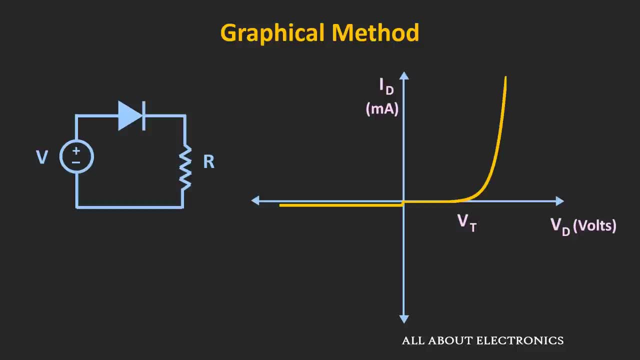 But first of all let's understand that. what is the load line? So here we have a very simple circuit in which some DC voltage is applied to this circuit and some current limiting resistor R is connected in series with this diode. Now here let's assume that the applied voltage is sufficient that it will forward bias. this 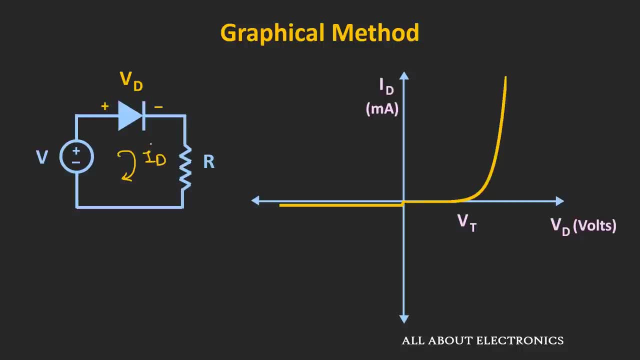 diode And let's assume that the voltage across this diode is equal to Vd and the current that is flowing through this circuit is equal to Id. So now, if we apply the KVL, then we can write this: voltage V is equal to Vd plus Id times this resistor R. 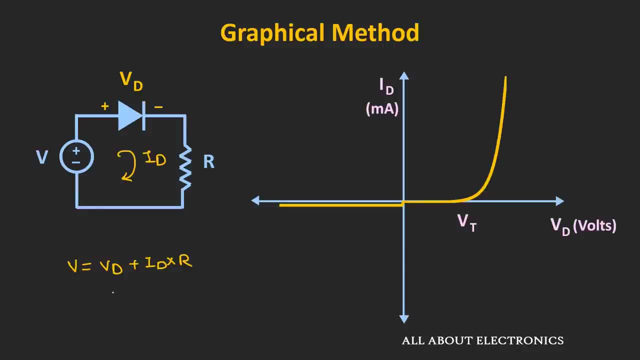 So if you see this voltage, V is equal to Vd plus Id times this resistor R. So if you see this equation, we have two variables: The voltage across this diode, Vd, and the current that is flowing through this diode. that is equal to Id. 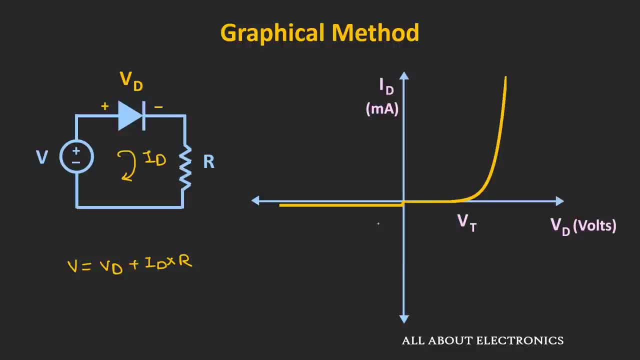 So from this expression we can find the line on this Id versus Vd curve and we can get the different possible values of Vd and Id. So, for example, if we put Vd is equal to 0, in that case we will get the extreme value. 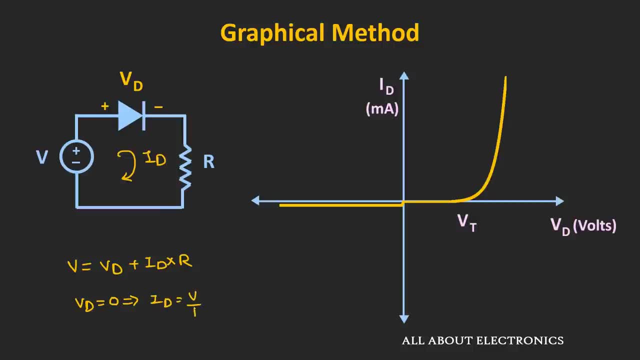 of this Id That is equal to V divided by R. So we will get one point on this y-axis That is equal to V divided by R. And similarly, if we put Id is equal to 0, in that case, we will get one point on this. 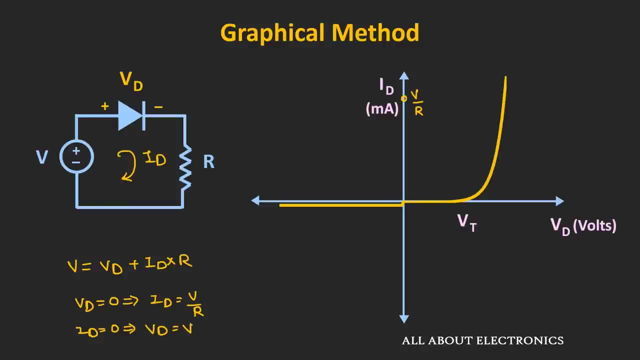 horizontal axis And that will be equal to Vd is equal to VV, So we will get one more point on this x-axis And by connecting these two points we will get the load line for the given circuit. So this intersection point will give us the 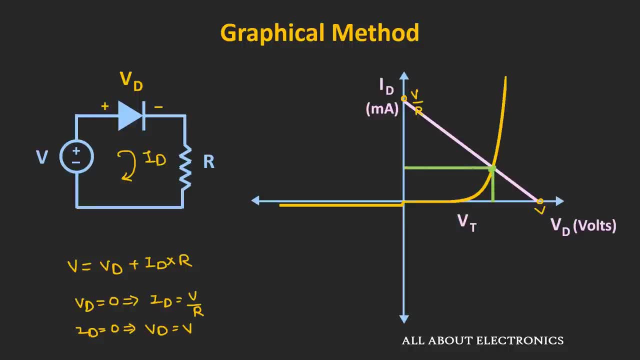 operating voltage and current for the diode. So in this way, using this load line, we can find the operating voltage and current for the diode. Although this graphical method gives us very accurate values of voltage and current, it is very time consuming process, So there is another way by which we can not. 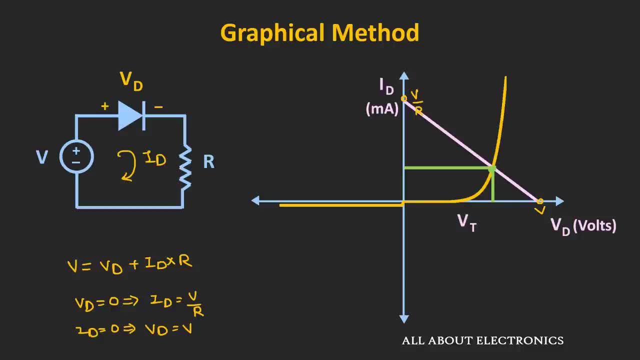 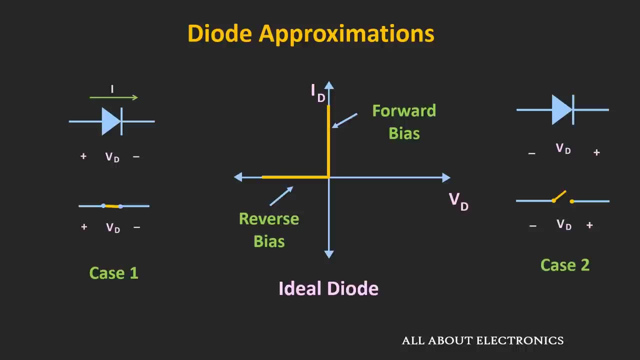 only quickly solve the circuits, but we can even troubleshoot the circuits, And this method is the diode approximation method. Now, in the introductory video of this diode we had seen the V-I character. This is the characteristic of the ideal diode. So if the diode is forward biased, in that 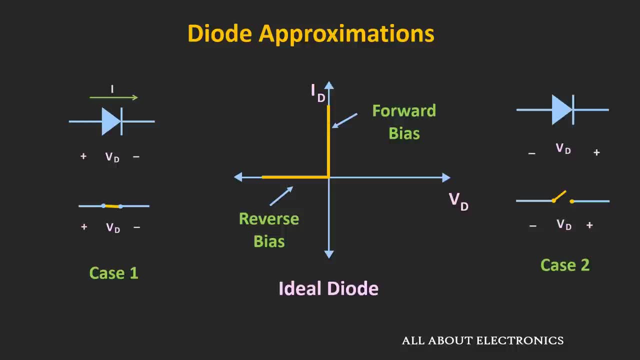 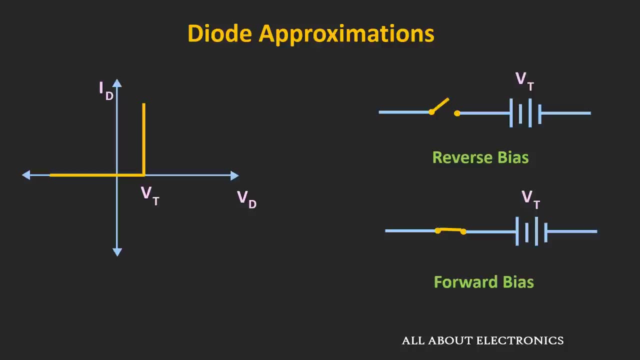 case, it will simply act as a closed switch. On the other hand, in case of reverse bias, it will act as an open switch. Then, after we had seen the second approximation, in which we had assumed that the diode will start conducting only when the applied voltage 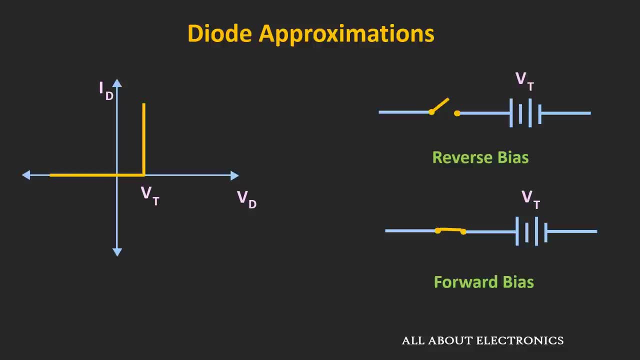 crosses some threshold voltage And if the applied voltage is less than this threshold voltage, in that case it will act as an open switch. Then, after we had also seen the third approximation, where we have also included some series resistance with this diode, Now in most of the circuits the current 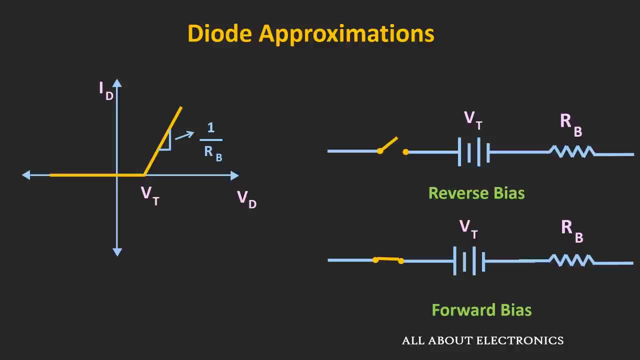 limiting resistor, which is connected in series with the diode, used to be much larger than the diode resistance, So in most of the cases we can neglect this diode resistance. So in our analysis we will use the second approximation, where we will assume that whenever the diode is forward biased, then the voltage 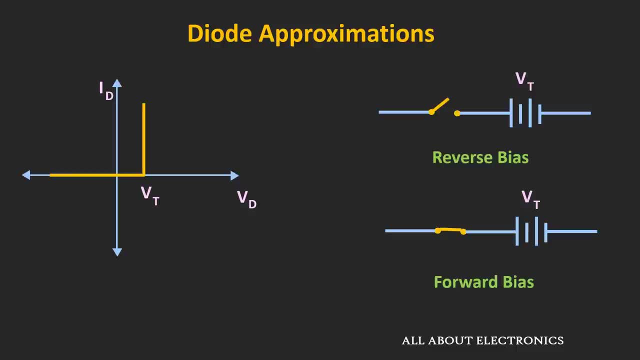 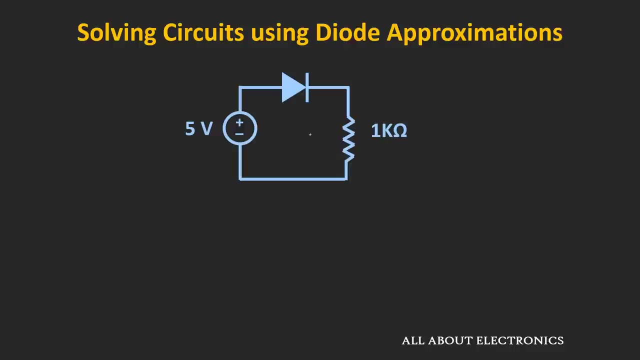 diode will be equal to 0.7V and whenever it is reversed, biased, then simply it will act as an open switch. So, using this approximation, let's solve some diode circuits. And let's start with very basic example. So in this circuit, a 5V of voltage is connected to this diode. 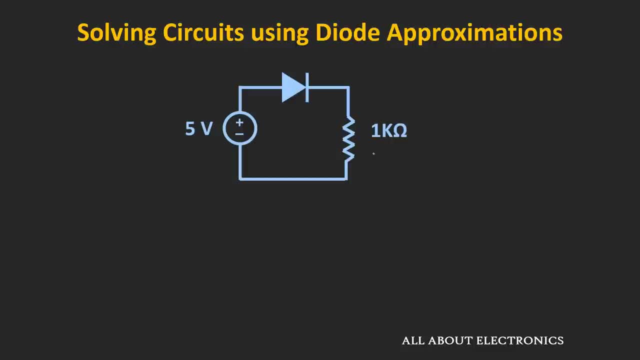 And here we also have a 1KΩ of current limiting resistor. So let's find out the voltage and current for the given circuit Now. first of all, we need to identify that whether this diode is conducting or non-conducting, 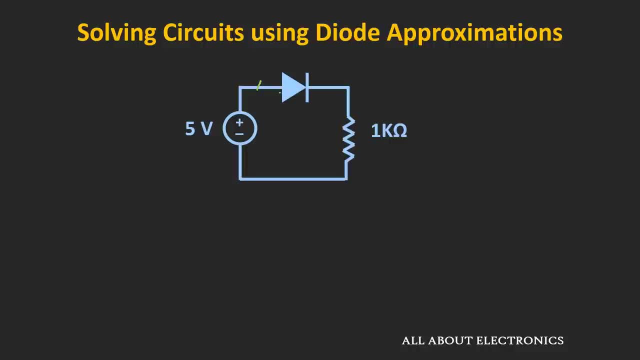 And that can be found by finding the Thevenin's equivalent voltage across this diode. Now here, if the applied voltage across this anodinth cathode of the diode is more than 0.7V, in that case we can say that the diode is conducting. 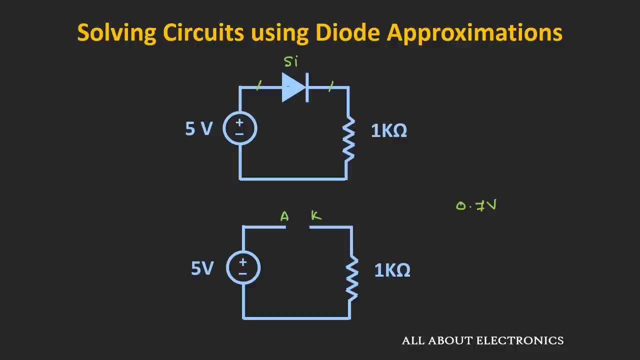 And here we are assuming that the diode that is connected is silicon diode. In case of a germanium diode, the threshold voltage is to be 0.7V. So in case of the germanium diode, the diode will start conducting whenever the applied. 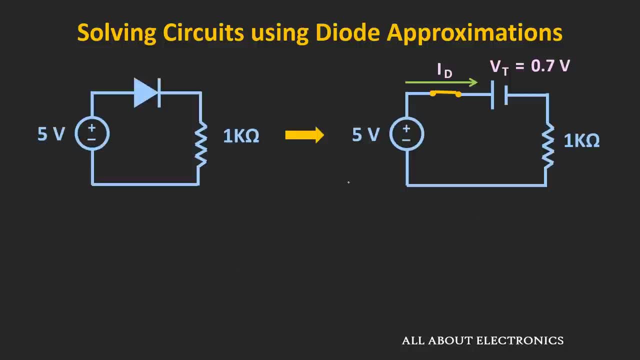 voltage across the diode is more than 0.3V. Now, here, as the diode is conducting, so let's represent it by its equivalent circuit, And here let's assume that the current that is flowing through the circuit is equal to Id. 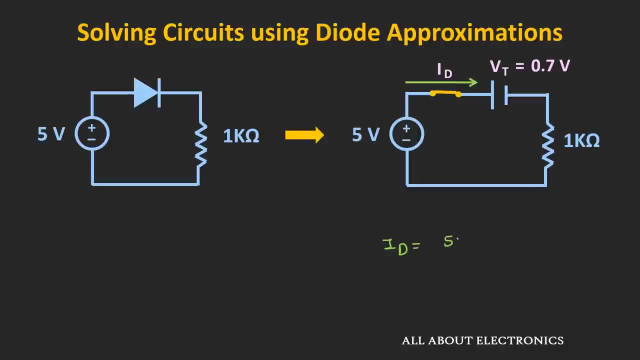 So this current Id will be equal to 5V-0.7V. divided by 1KΩ, That is equal to 4.3mA. So this is the current which will flow through this particular circuit And the voltage across the diode will be equal to 0.7V. 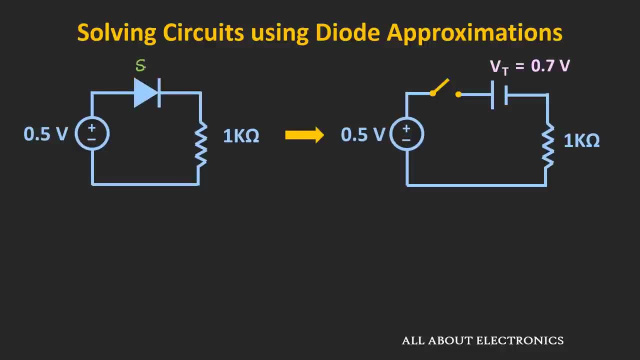 Now in this circuit. if we assume that the diode that is connected is silicon diode and the applied voltage is 0.5V, in that case it will not cross the barrier of this silicon diode, So the circuit will act as an open circuit. 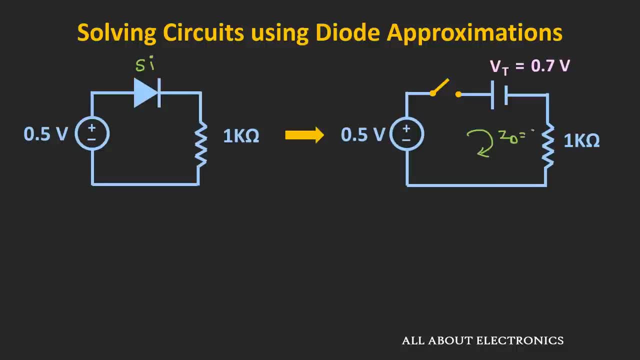 And hence the current that is flowing through the circuit will be equal to 0.7V-0.7V. But instead of silicon diode, suppose we have a germanium diode. in that case this diode will conduct. So, as you can see, in case of the germanium diode this circuit will conduct, while in 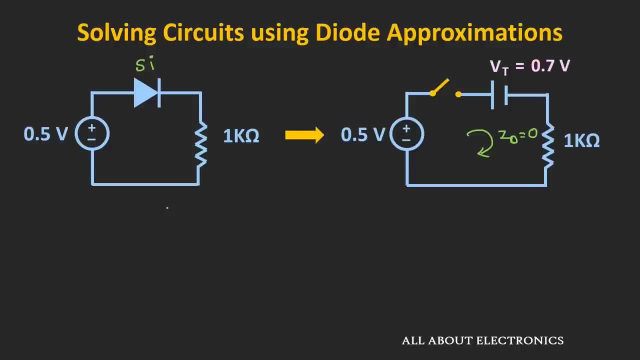 case of the silicon diode, this circuit will act as an open circuit. So while solving the circuits, we also need to see the type of diode which is connected in the circuit. Alright, so now, once again, let's assume that the diode that is connected in the circuit 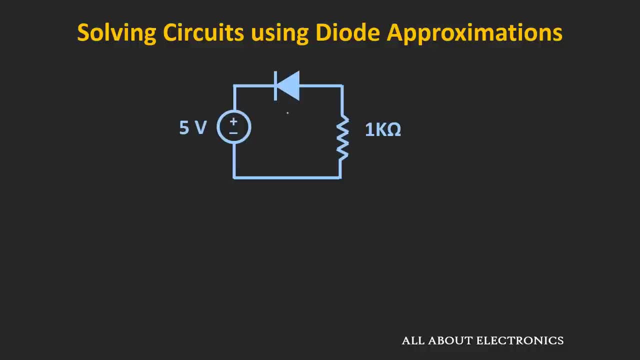 is silicon diode. However, the direction of the diode has been reversed. So in this case, if you see, if you find the Thevenin's equivalent voltage, then now, across this anode and cathode, the voltage will be equal to minus 5V. 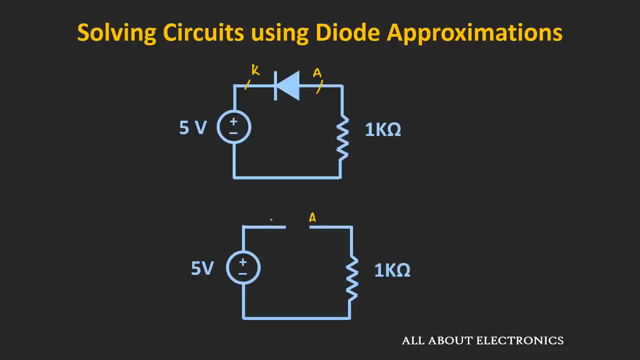 Because now the anode is on the right hand side and the cathode is on the left hand side, So equivalent voltage across this diode will be equal to minus 5V, And hence this diode is reversed bias, So there will not be any flow of current in the circuit. 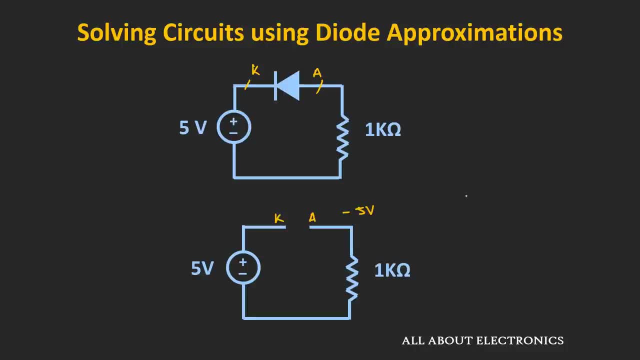 And hence this diode is reversed bias, So there will not be any flow of current through this circuit And simply we can say that this diode current Id will be equal to zero. So, as you can see, using this diode approximation, we can easily analyze and solve the circuit. 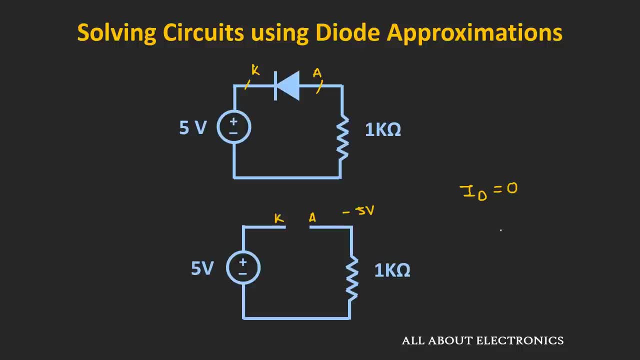 problems Now using this approximation. the values of the voltage and current that we have got are not accurate values, but they are quite close to the actual values. So for analyzing or troubleshooting the circuits we can use this diode approximation. Alright. 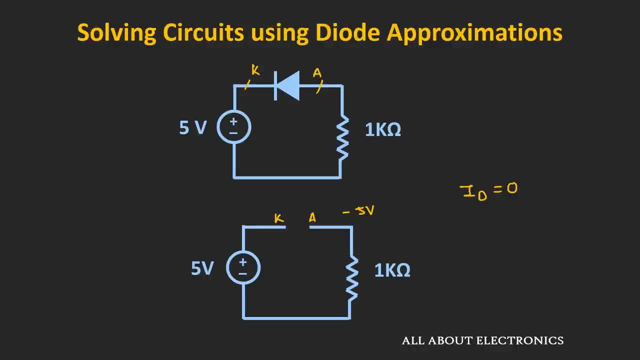 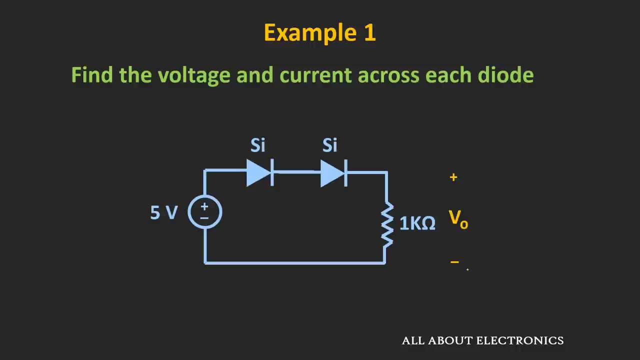 So now let's see few more examples based on these diode circuits. So in this example, the two silicon diodes are connected in series and we have been asked to find the voltage and current across each diode, as well as we have been asked to find 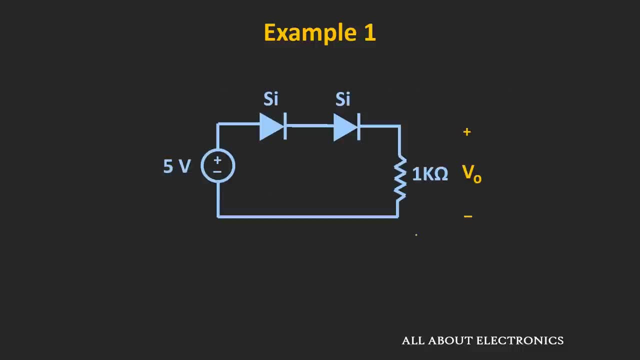 the output voltage across this 1kΩ resistor. Now, for a moment, let's assume that these two diodes are conducting and, as they are silicon diodes, so in case of the forward bias, the voltage across each diode will be. 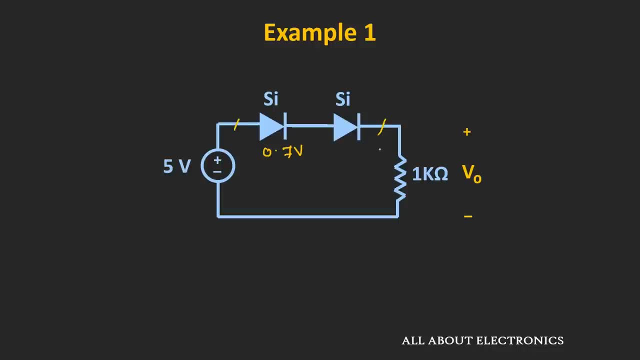 equal to 0.7V. So to turn on these two diodes, the voltage across the two terminals of this diode pair should be more than 1.4V, And here, as the applied voltage is 5V, so these two diodes will turn on. 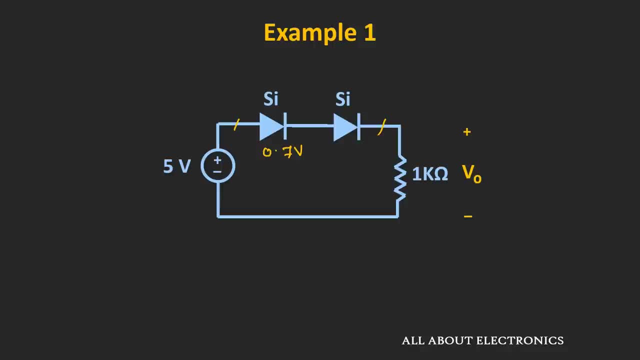 So let's replace these two diodes by their equivalent circuit, And if you see the equivalent circuit, then it will look like this. Now, here, let's assume that the current that is flowing through the circuit is equal to I, So the current I can be given as 5 – 0.7 – 0.7, and that is divided by 1kΩ resistor. 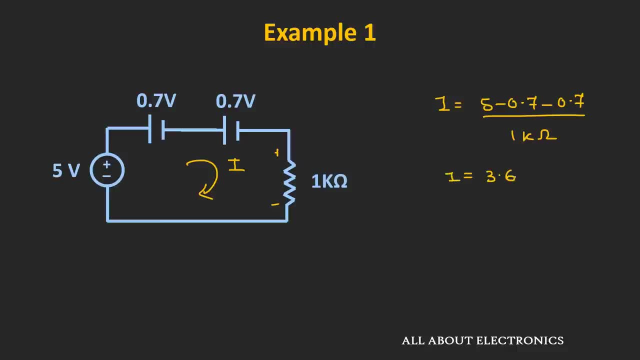 So the value of this current I will be equal to 3.6mA. Now the output voltage Vout will be the drop across this 1kΩ resistor. So the output voltage Vout will be equal to 3.6mA multiplied by 1kΩ resistor. 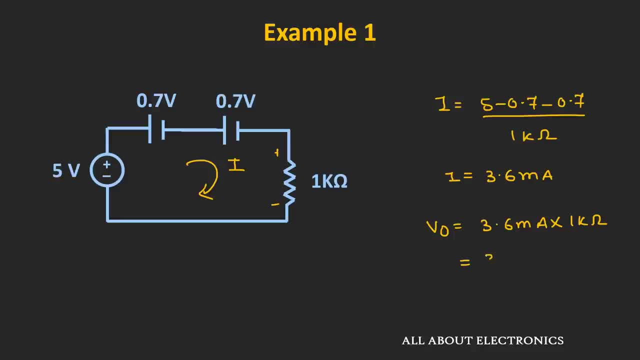 So the output voltage Vout will be equal to 3.6mA multiplied by 1kΩ resistor. out across this 1kΩ resistor will be equal to 3.6V. So in this way, in case of the series connection of the diode, the threshold voltage to turn 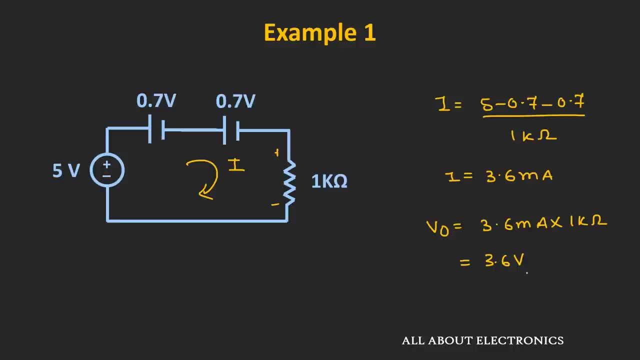 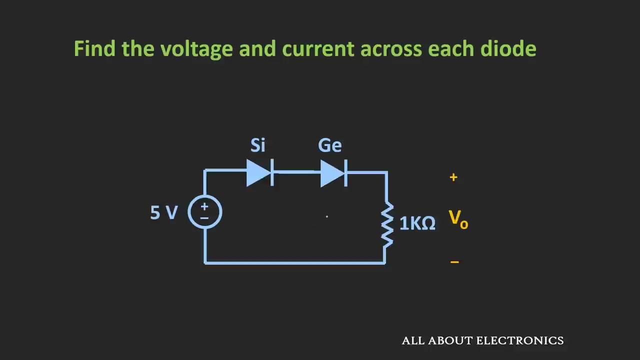 on the diode will increase. So, instead of the 2 silicon diodes, if we have 3 silicon diodes which are connected in series, the threshold voltage to turn on this diode will increase to 2.1V. So, similarly, try to find the current and output voltage in the given circuit. 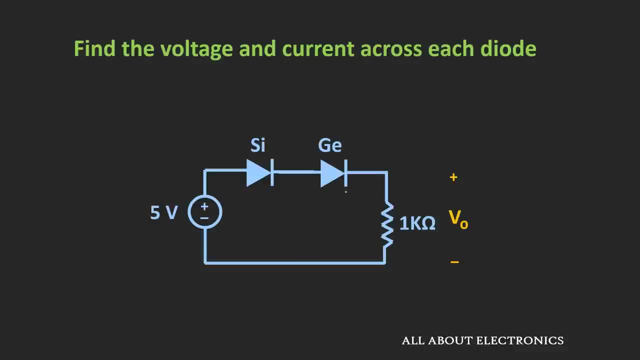 Now, this circuit is similar to the previous circuit, but here one silicon diode is replaced by this germanium diode. So try to find the answer and do let me your answer in the comment section. Alright, so now let's move to the next example. 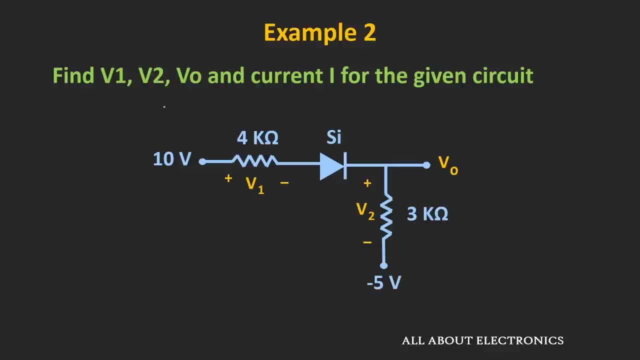 So in this example we have been asked to find the value of these voltages V1, V2 and Vout. Now, if you see the circuit, the anode of this diode is connected to the 10V through this 4kΩ resistor. While the cathode is connected to the 4kΩ resistor. Now, if you see the circuit, the anode of this diode is connected to the 10V through this 4kΩ resistor, While the cathode is connected to the 4kΩ resistor. 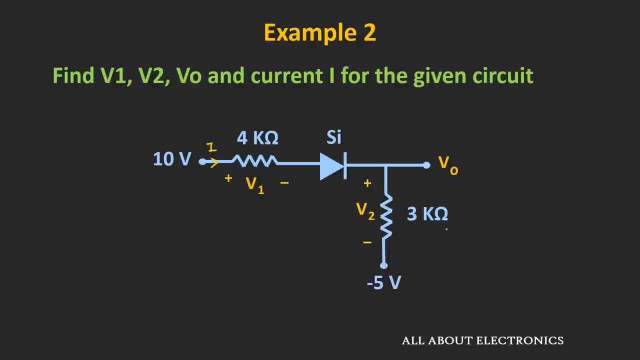 As you see, the electrical circuit is connected to the 5V through this 3kΩ resistor, So intuitively you can say that this diode will turn on. So here, if we apply the KVL, then we can write 10 minus V1 minus 0.7V. that is the drop across. 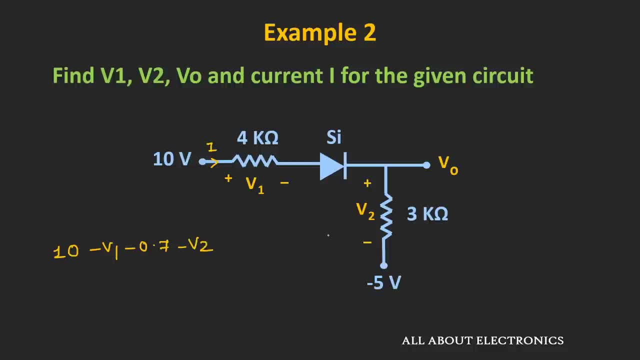 this silicon diode minus V2, that is the drop across this 3kΩ resistor- minus minus 5V, And that will be equal to 0. So if we simplify it, then we will get 14.3V. that is equal to V1 plus V2.. 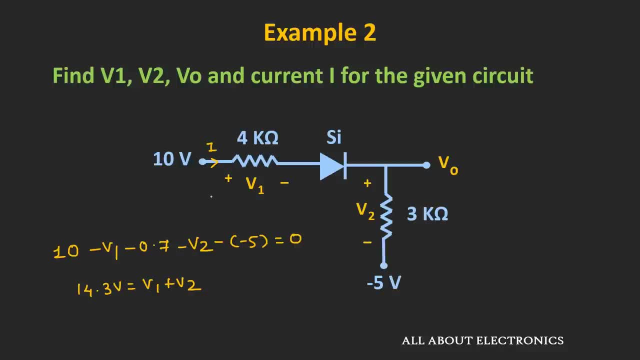 Now here we have assumed that the current that is flowing through this circuit is equal to I, So this V1 will be equal to 4kΩ times this current I, And this V2 will be equal to 3kΩ times this current I. 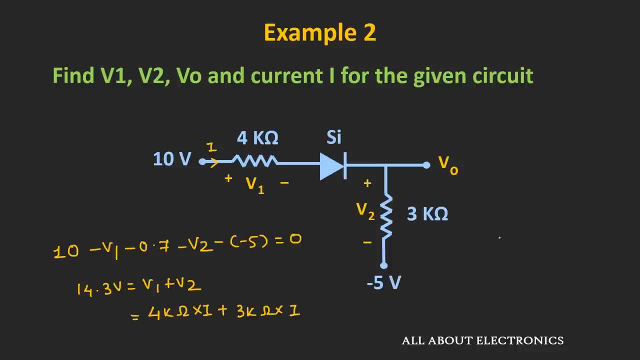 So if we simplify it, then we can say that this current I will be equal to 14.3V. divided by 7kΩ, That is roughly equal to 2.04 mA. So this is the current which will flow through this circuit. 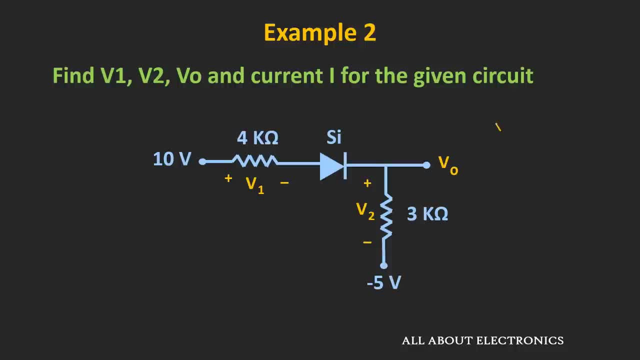 So from this we can say that this voltage, V1 will be equal to 4kΩ. multiplied by this current I, That is equal to V2. 8.16V. And similarly, V2 will be equal to 2.04 mA multiplied by 3kΩ. 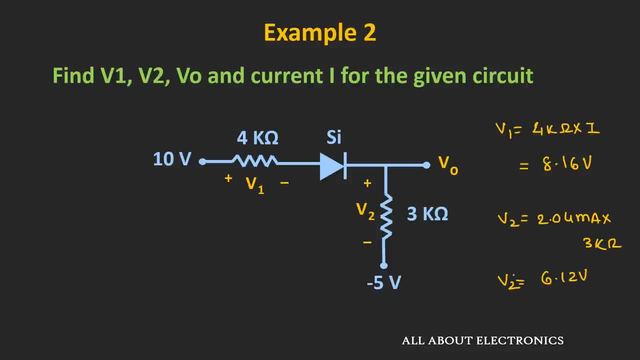 That is equal to 6.12V. So these are the values of voltage V1 and V2.. Now here the output voltage Vout will be equal to V2 minus 5V, That is equal to 6.12V minus 5V. 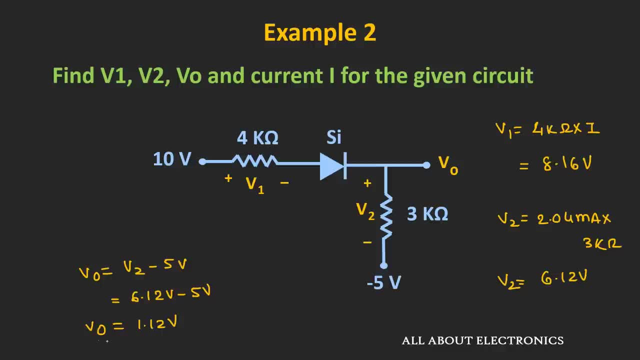 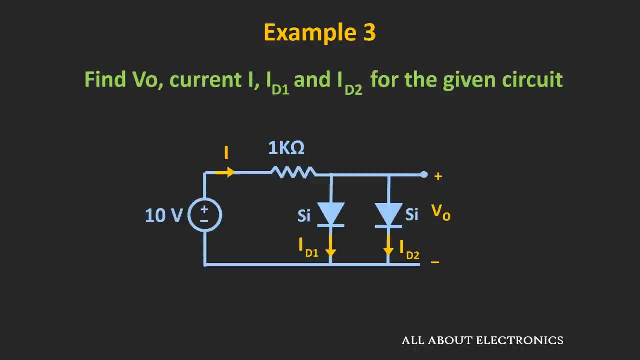 And that is equal to 1.12V. So this is the actual value of the output voltage. Alright, so now let's move to the next example. Now, here, these two diodes are connected in the parallel connection And we have been asked to find the value of the output voltage as well as the current. 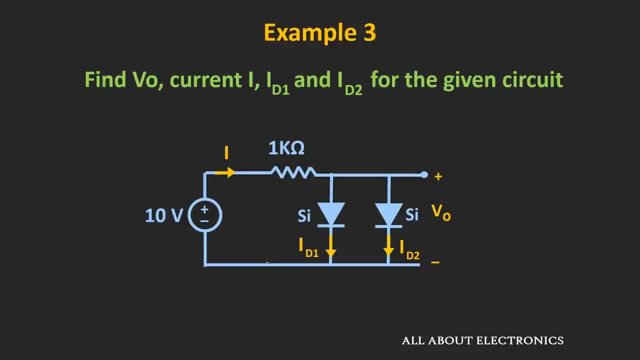 I that is flowing in the given circuit, And we have been also asked to find the value of the diode currents Id1 and Id2.. Now, if you see this circuit here, the two terminals of these diodes are connected to the ground potential. 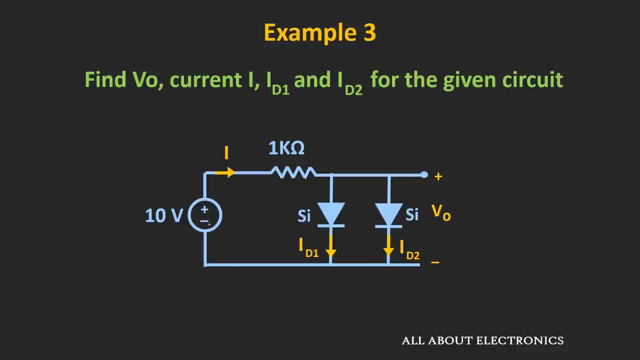 And the anode of these two diodes are connected to the 10V through this 1kΩ resistor. It means that these two diodes will become forward biased. It means that the output voltage which we will get across these two diodes will be equal. 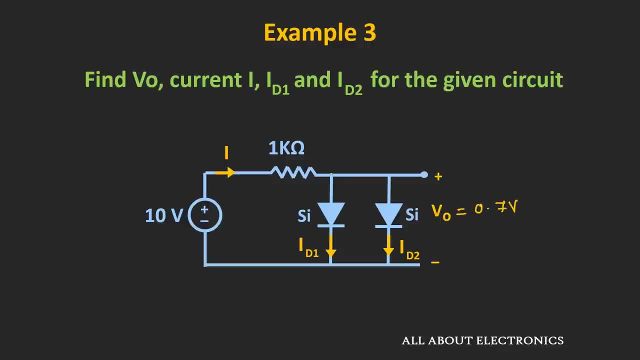 to 0.7V. It means at this node the voltage is equal to 0.7V. So from this we can easily find the current that is flowing in the circuit. So the current I will be equal to 0.7V. 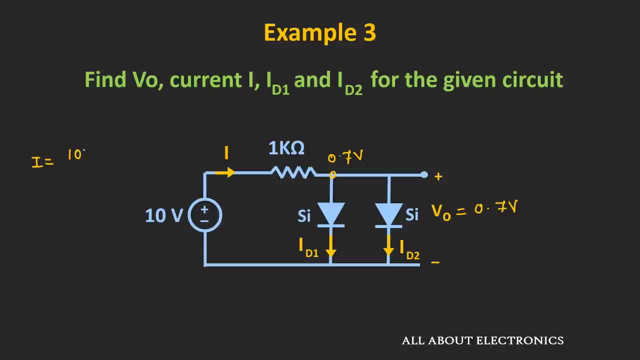 So the current I will be equal to 0.7V. So the current I will be equal to 0.7V. 10V minus 0.7V divided by 1K ohm resistor And that is equal to 9.3 mA. 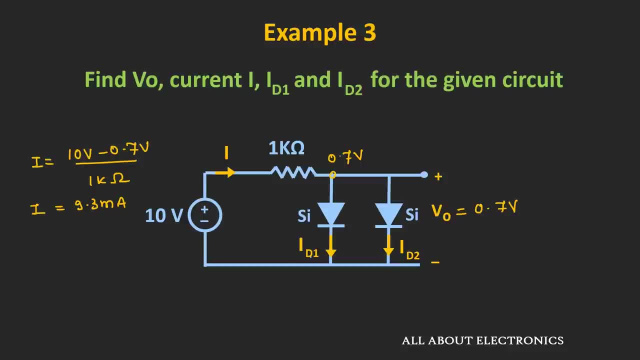 So this is the total current which will flow in the given circuit. Now here we are, assuming that these two diodes are identical, So this current I will get equally divided between the two diodes. It means that the current ID1 and ID2 will be equal to 4.65 mA. 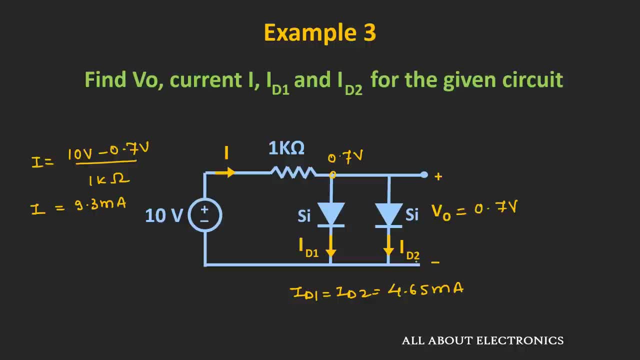 Now in this example, as the two diodes which are connected in parallel are identical, so it is easy to solve this particular problem. But if the two diodes which are connected in parallel are made up of different materials, then we need to see the threshold voltage of each diode. 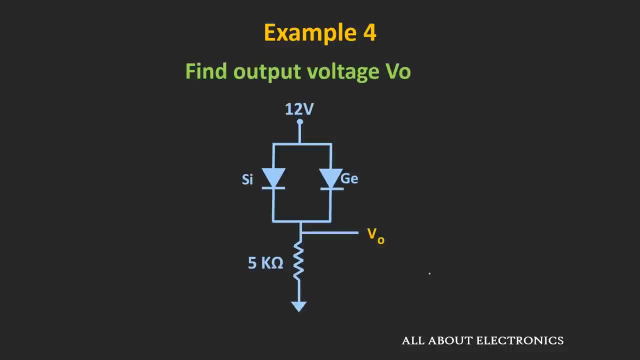 So based on this, we will see the next example. So in this example the silicon and the germanium diodes are connected in the parallel connection. Now, here for a moment, let's assume that the two diodes are conducting simultaneously, And first of all let's assume that this silicon diode is conducting. 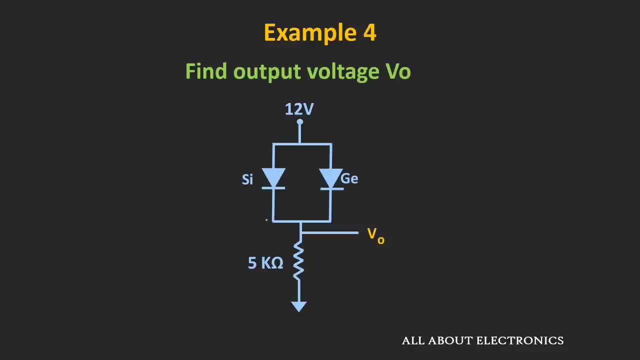 So if this silicon diode is conducting, then there will be a voltage drop of 0.7 across this diode. So at this node the voltage will be equal to 12 minus 0.7.. That is equal to 11.3V. 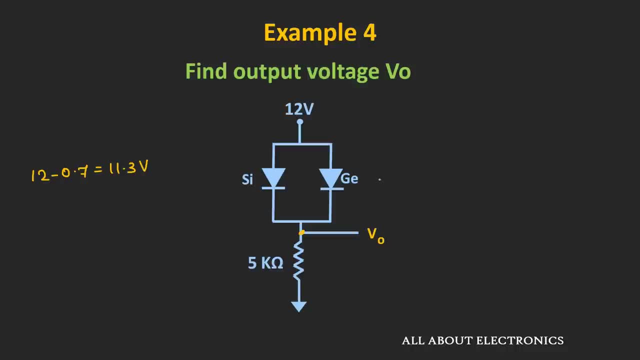 Now let's see the next example. Similarly, let's assume that this germanium diode is also conducting. So if this diode is conducting, then the voltage drop across this diode should be equal to 0.3V And the voltage drop across this silicon diode should be equal to 0.7V. 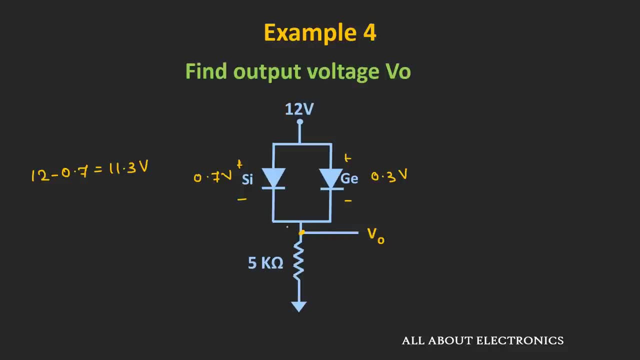 Now, as these diodes are connected in the parallel connection, the voltage drop in the parallel connection should remain constant. But here the one diode has a voltage drop of 0.7V, while the other diode has a voltage drop of 0.3V. 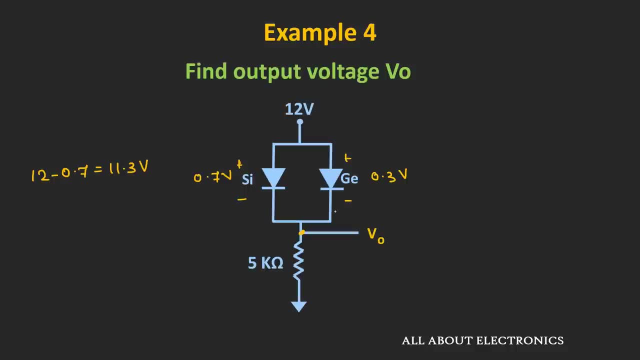 It means that only one diode should conduct and one diode should remain off. So let's find out which diode will conduct and which diode will remain off Now in this circuit, whenever the 12V voltage is applied to these diodes. in reality, this: 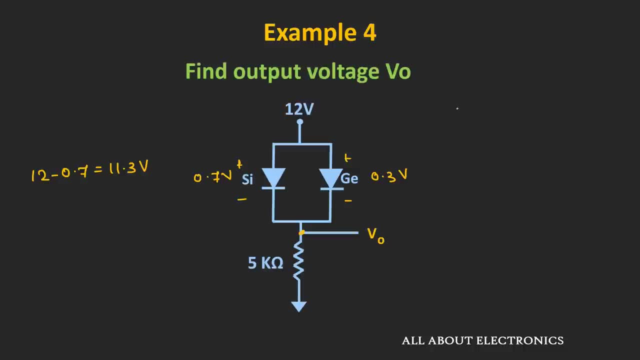 voltage will take some time to reach from 0 to 12V Now, during the course of this transient, if you see first of all, this germanium diode will turn on. It will try to maintain the voltage across the two terminals. 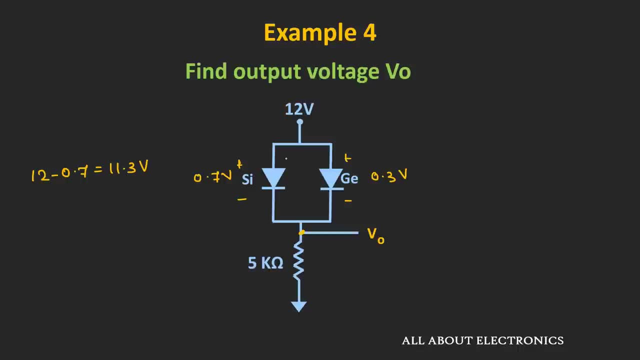 So, because of that, this voltage across the silicon diode will also remain 0.3V And hence this silicon diode will not be able to turn on. So, if you see, actually the voltage across the two terminals will remain 0.3V. 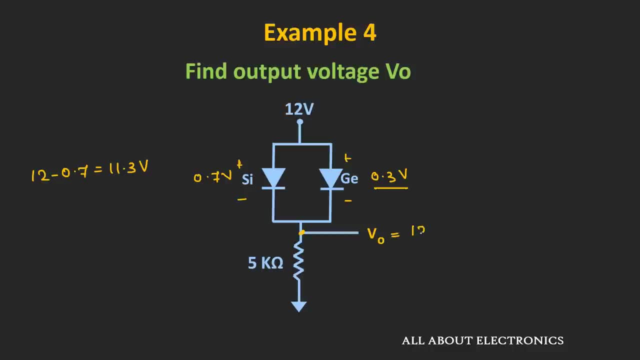 So the output voltage Vout in reality will be equal to 12V-0.3V, That is equal to 11.7V. So in this way, whenever the two different types of diodes are connected, the voltage of diodes are connected in parallel. then we need to see the threshold voltage or the 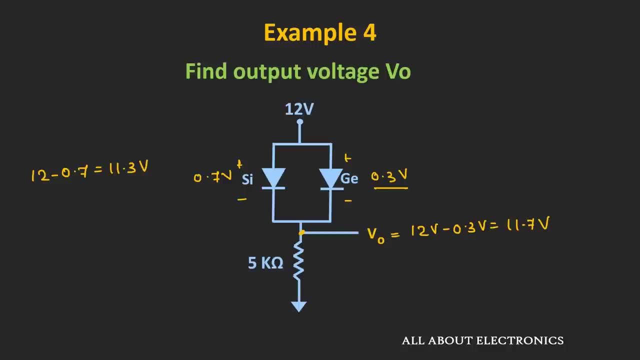 cut-in voltage for each diode. So the diode which has a lower cut-in voltage will turn on first. Alright, so based on this, let's see the last example Now. in this example also, we have been asked to find the output voltage. 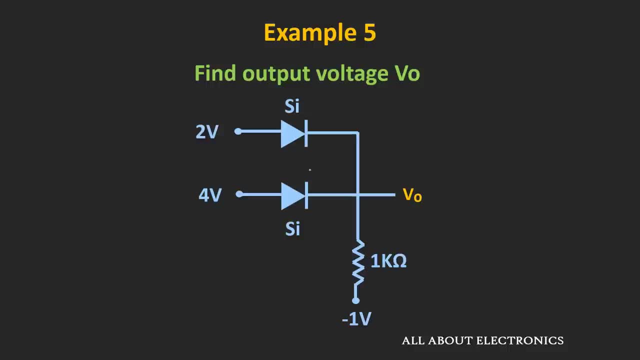 Now here to find the output voltage. let's assume that both diodes are conducting simultaneously, And first let's talk about the first diode. So if the first diode is conducting, Then the voltage at this node should be equal to 2V-0.7V. 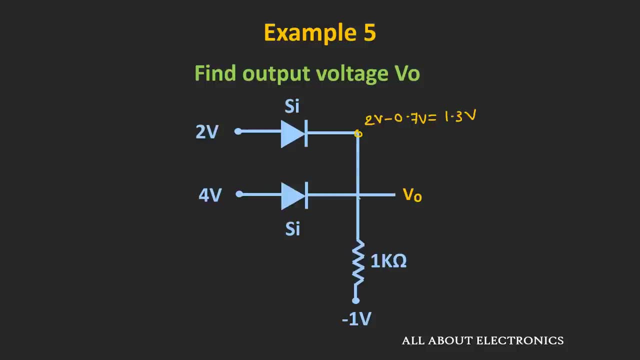 That is equal to 1.3V. Now the same voltage will also appear at the cathode of this second diode, And the anode of the second diode is connected to the 4V. It means that the second diode will also become forward biased. 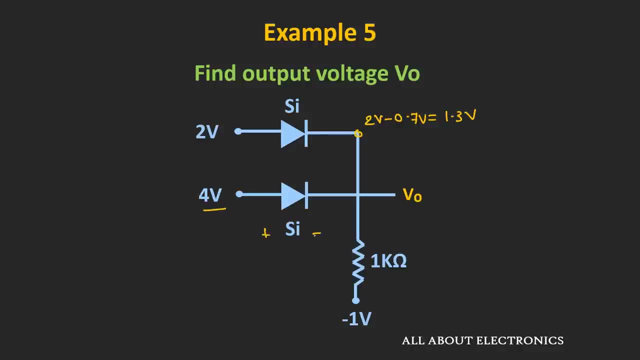 And if this diode is turned on, then there will be a 0.7V of voltage drop across this diode. So if we consider this second diode as a conducting diode, Then the voltage at this node should be equal to 4V-0.7V. 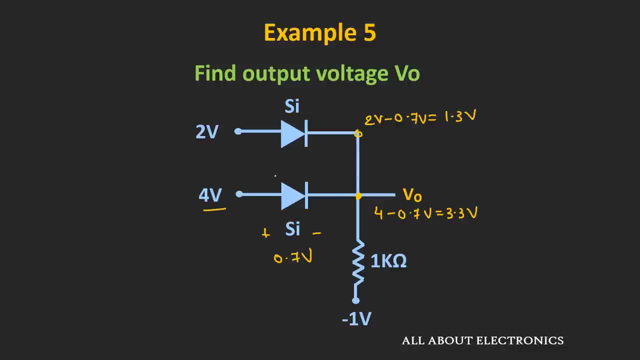 That is equal to 3.3V. But here, if both diodes are conducting simultaneously, then you can see that there is a contradiction at this node. It means that both diodes cannot conduct simultaneously. Now suppose if we assume that this second diode is conducting only. 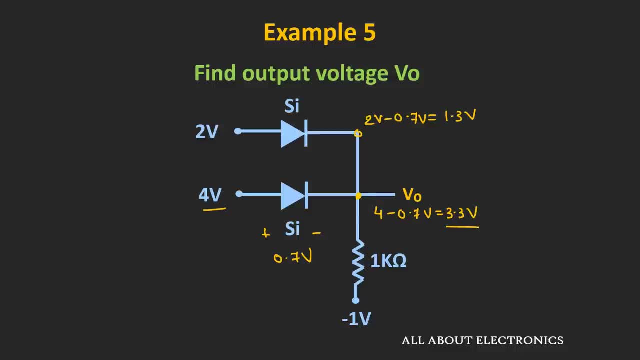 In that case the voltage at this node will be equal to 3.3V, And at this node also The voltage should be equal to 3.3V. So if this is the case, then the first diode will remain OFF. 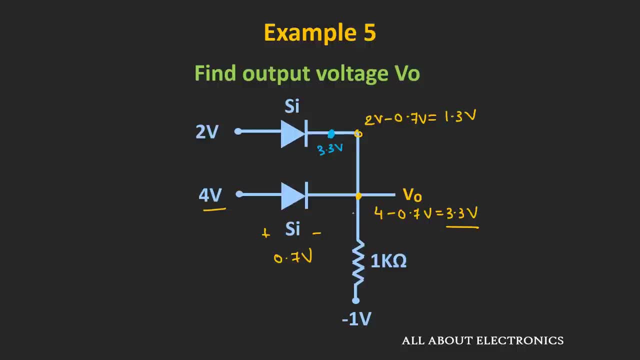 And there will not be any contradiction of the voltage. So it means that the assumption that we have made is correct. That means the first diode will remain OFF And the second diode will remain ON, And the actual voltage at this node will be equal to 4V-0.7V. 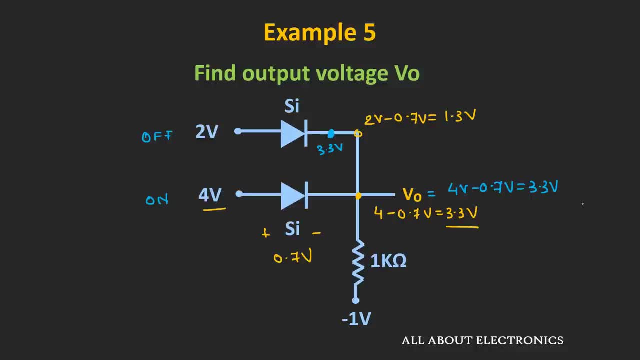 That is equal to 3.3V, So this is the output voltage for the circuit. So I hope in this video you understood how to solve the problems based on the diode And we will solve some more examples in the upcoming quiz.